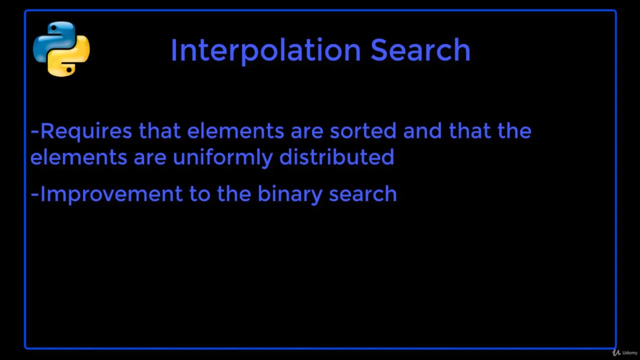 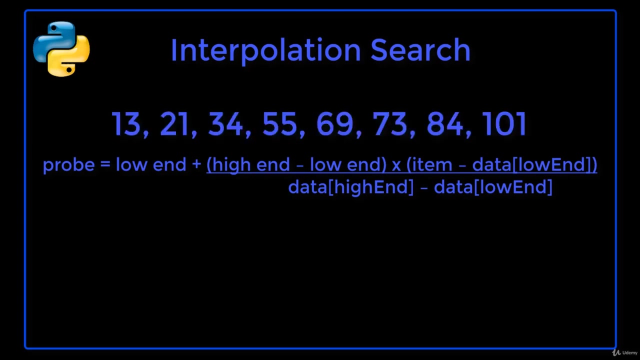 it doesn't always start in the middle. If it is looking for an element closer to the beginning, it will start closer to the beginning, and vice versa. The only difference between a binary search and an interpolation search is the calculation of the probe position. The formula for calculating the probe position is the following formula: 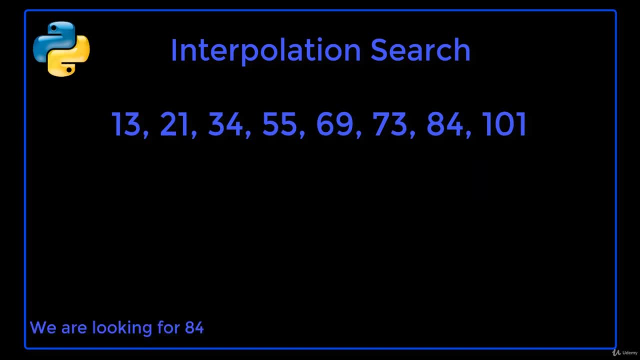 Here is the collection of example data that we will be using for this example. We will be searching for element 84.. The first step is to calculate the position of the probe. This results in 5.6.. The .6 gets chopped off, leaving us with 5 as the probe position. 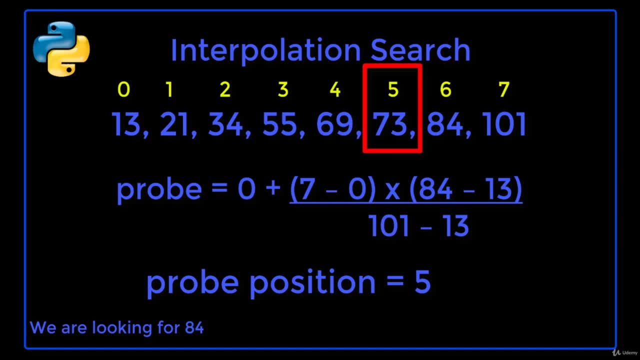 Therefore, the probe is 73, the element at index 5 in the collection 84, the element we are searching for is greater than the probe 73.. Per the algorithm, the low end will become the probe plus 1, meaning 84 is now both the 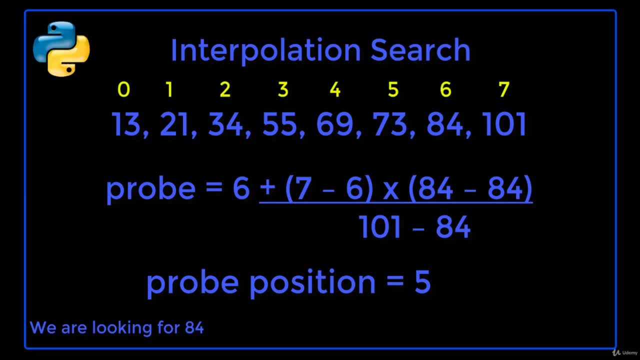 low end and the probe 101 will be the high end. Now we plug the new numbers into the formula and get 6, the exact index of 84, the element we are searching for. Now that we have a conceptual understanding of what an interpolation search is, let's 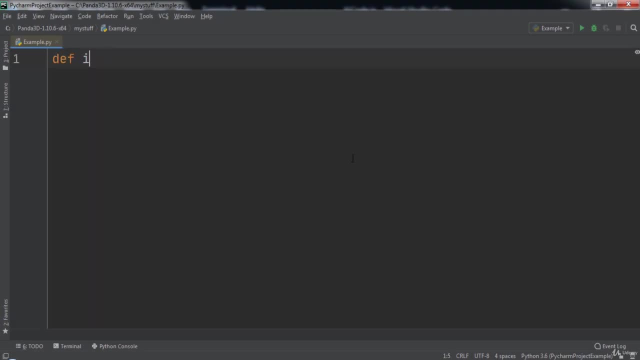 write the Python code to implement the logic. We will use the def keyword and name our function: interpolation search. It will take in two parameters: elements, which will be the list of elements we are searching through, and x, the element we are searching for. 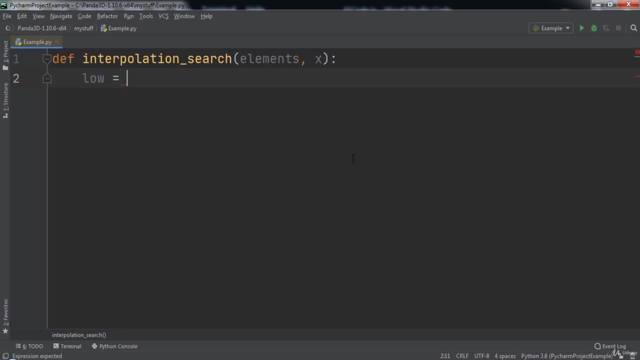 Inside of our function, we will have a variable named low, set equal to a value of zero. Then we will have a variable named high, set equal to the length of elements minus one, While While low is less than or equal to high and x is greater than or equal to elements at. 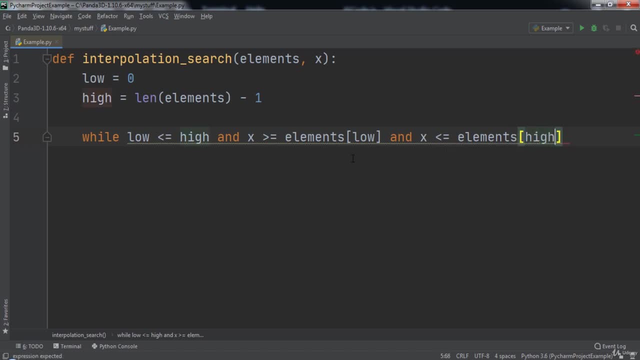 low and x is less than or equal to elements at high, we will check if low equals high. If so, we will check if elements at low equals x. In that case we will return low, else we will return negative 1.. 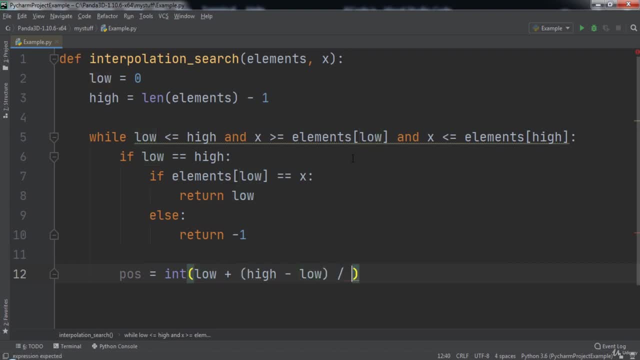 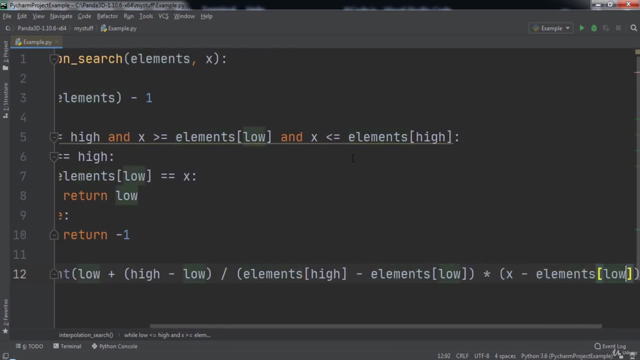 Then we need to plug in that formula that we used to find the probe position. This is the formula that we just went over in the conceptual example. Please type it in exactly as you see me typing it here. Then we will check if elements at the position equals x, the element we are searching for.